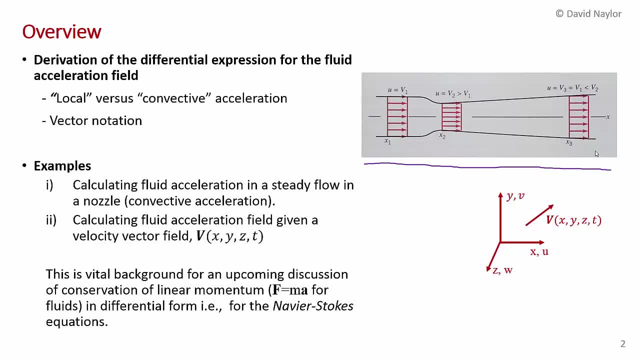 So the next question is vital background for the next video where I discuss the conservation of linear momentum. What we're going to discuss in the next video is basically F equals M, A or Newton's Second Law for fluids. It's the conservation of linear momentum in differential form and that yields the Navier-Stokes equations which I mentioned in the first video of Chapter 4.. 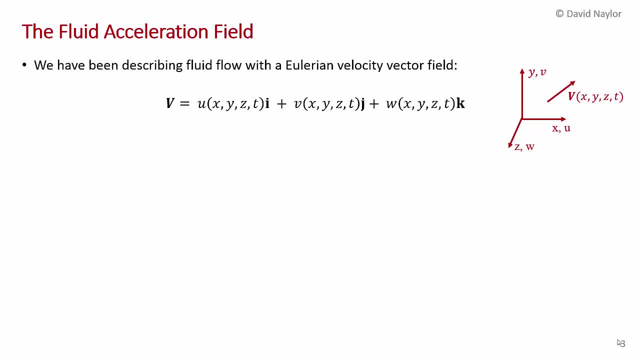 Which I mentioned in the first video of Chapter 4.. So, as we have been discussing these equations, I'm going to start by focusing on the linear momentum. So, as we have been discussing these equations, I'm going to start by focusing on the linear momentum. 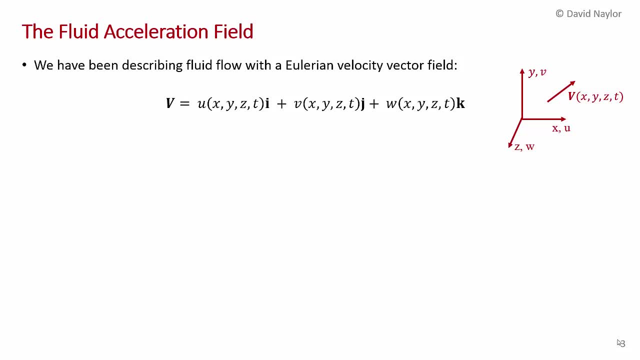 So, as we have been doing so far in the course, we're going to describe the fluid flow with an Eulerian vector field. So our velocity vector v has three components: u in the i direction, v in the j direction and w in the k direction. 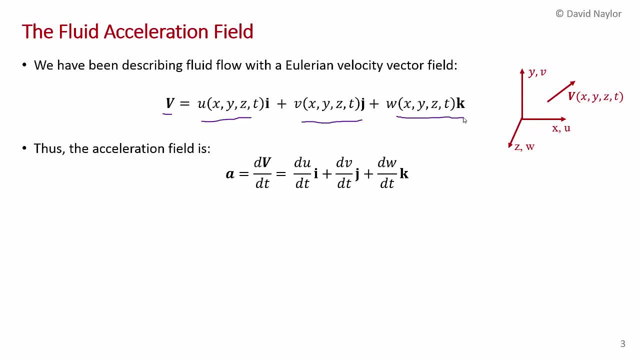 So if we take the derivative of this velocity vector, we end up with three components of acceleration. We end up with du dt in the i direction, dv dt in the j direction and dw dt in the k direction. But we have to note that each velocity component, uv and w, are functions of four variables. 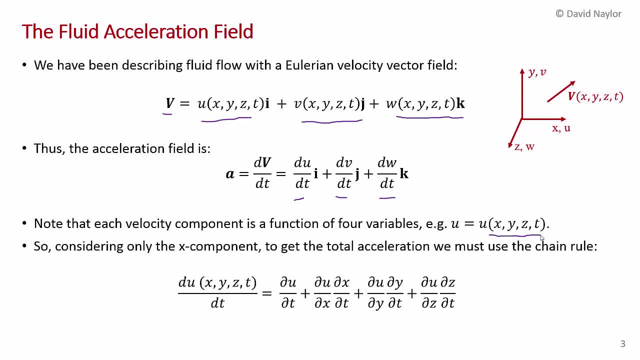 For example, u is a function of the three spatial coordinates and time. So if we want to get the total acceleration we've got to use the chain rule. And down at the bottom I've I've just considered the x component. so just considering u, the x component of velocity. 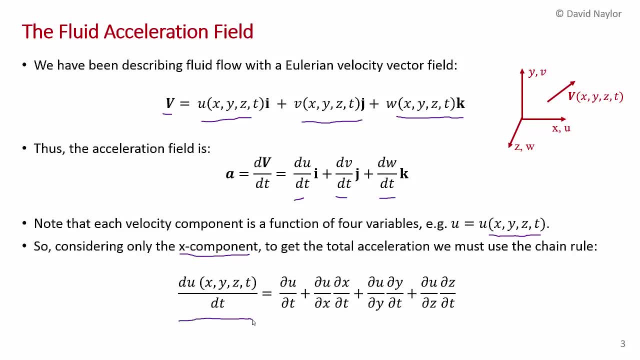 If you want to get the total acceleration, then you've got to consider the partial derivative of u with respect to t, the partial derivative of u with respect to x, then dx, dt, using the chain rule: du dy then dy dt and du dz and dz dt. 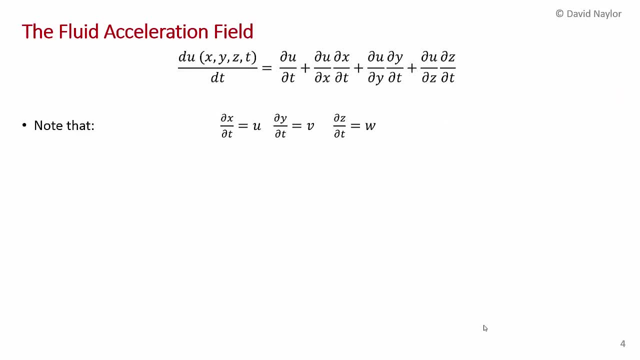 So what I've done, What I've done on the next slide, I think I've just rewritten this- So that's our total acceleration, considering the fact that u is a function of x, y, z and time. But these components, dx, dt is just the u component of velocity here. 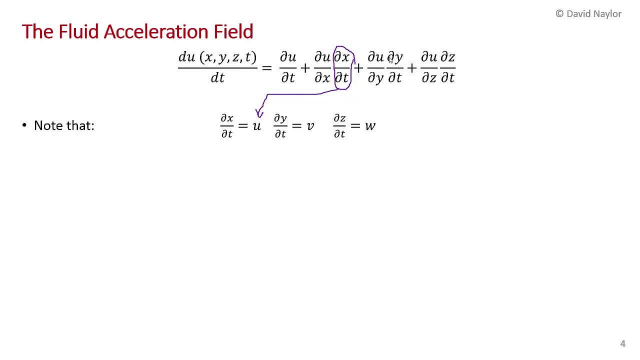 So the rate of change of x with time is u, the rate of change of y with time here is v, and the rate of change of z with time here is v, And that is just the w component of velocity. So now we can make those substitutions and it'll become u, v and w for those terms. 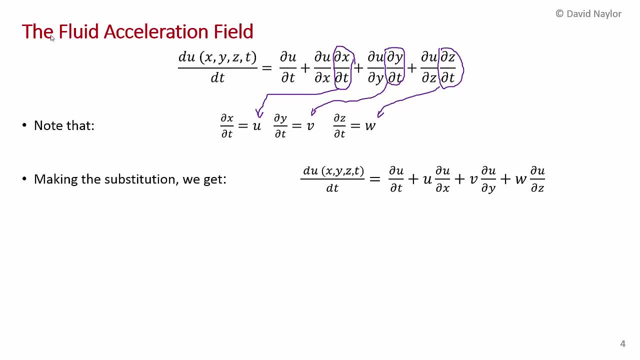 And so making the substitution now our total acceleration, and all we're considering again is the x component of velocity for the moment. so the acceleration in the x direction, The total acceleration is du dt plus u, du dx, v, du dy, w, du dz. 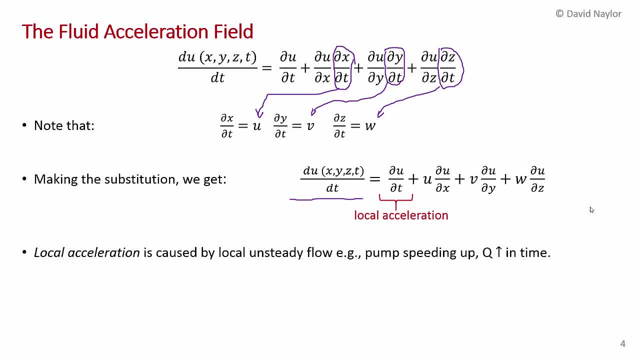 And, as I mentioned in the introduction, there are sort of two types of acceleration that we have to worry about. One is the local acceleration, That would be du dt for the u component of velocity, And that's, for example, if you have a transient flow. 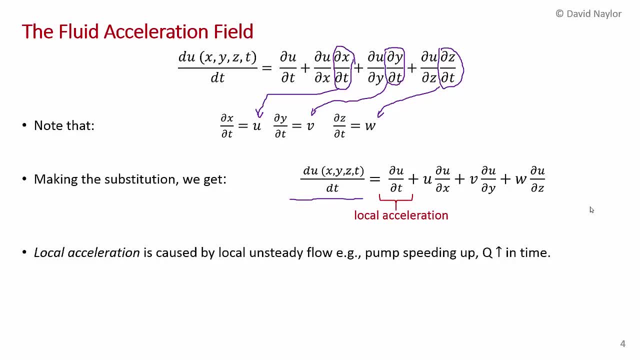 So if the pump is speeding up and you've got the flow rate increasing in time, the velocity at a point is going to be increasing with time. So at x, y, z, at a given spot, the velocity is going to be increasing as a function of time. 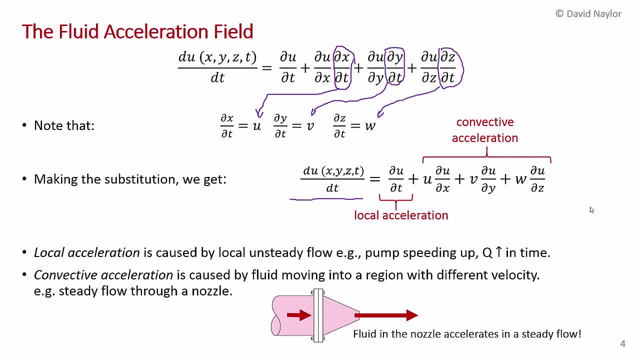 But then, in addition, you've got these convective acceleration terms that I alluded to when I talked about the Venturi tube. These local acceleration tubes- u du dx, v du dy and w du dz- are caused by the flow moving into a zone of higher velocity. 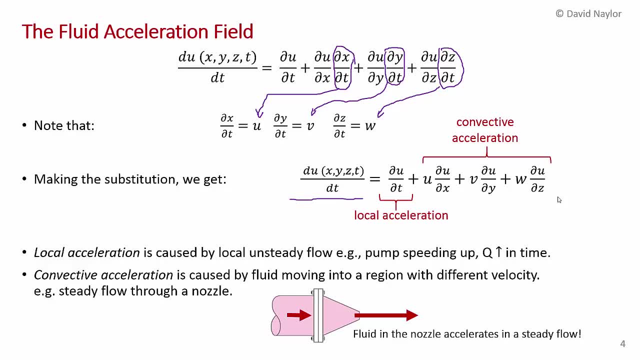 And you've seen this in, for example, steady flow in a nozzle or in a Venturi. The flow enters at low velocity but exits at high velocity. So even in a steady flow you have accelerations, And those accelerations are described by these convective terms over here. 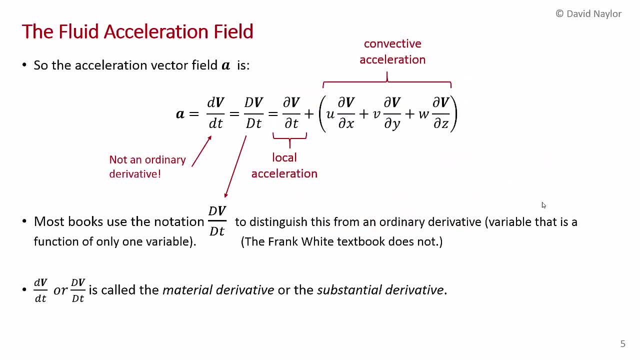 The previous slide, I only considered the u component of velocity. If you take that same idea, but you apply it to the acceleration field and to the velocity vector v whenever I bold something, by the way, just to remind you, just as the text. 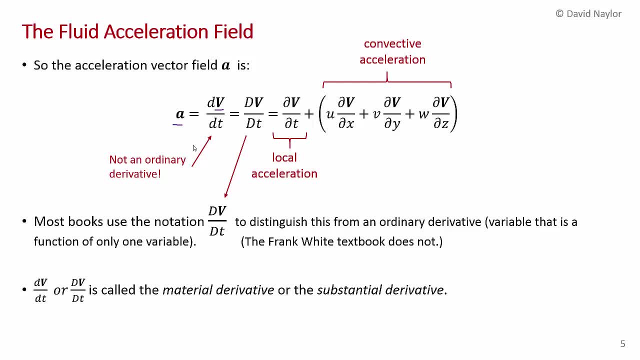 whenever you have something that's bold, that's a vector, And so if you apply that same concept to the acceleration field, to the acceleration vector, you get this expression here, where I've simply replaced in. here, instead of having u, I have the three components of the velocity vector. 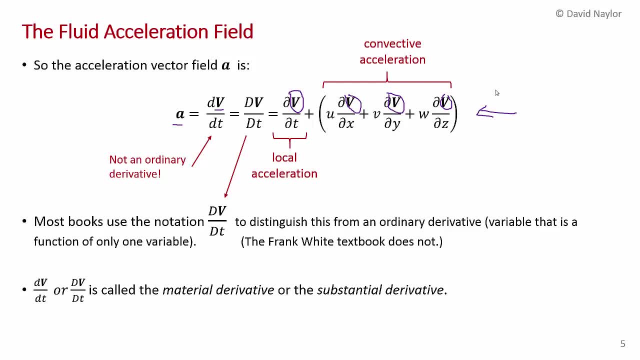 So this acceleration field is is denoted in your book as dv, dt. here It's this derivative. Now that's a little bit confusing because it looks like an ordinary derivative. It looks like v is a function of only one variable. Frankly, I don't like the way the white textbook does that. 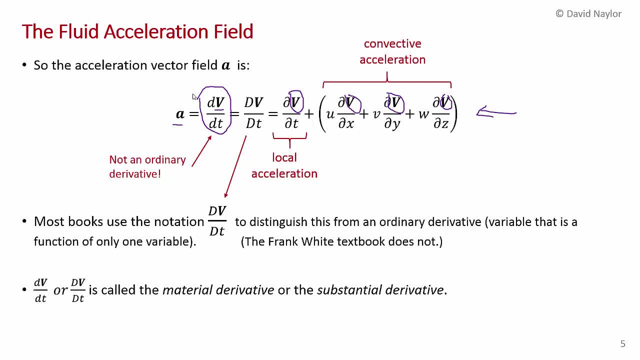 Most other books don't use a lowercase d there. They use an uppercase D to distinguish that kind of derivative from an ordinary derivative. So you'll have to be a little bit flexible and notice this in your book, This kind of derivative where you include the local and convective accelerations. 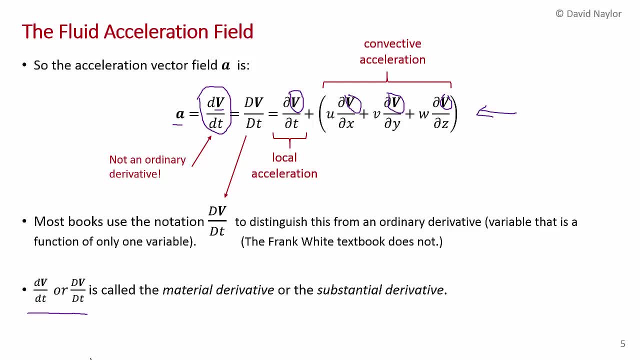 is called the material derivative or the substantial derivative or, in some books, the substantive derivative, And so it's different. It's not an ordinary derivative. v is a function of, of course, three spatial coordinates in time, So you have to keep your eye out for that. 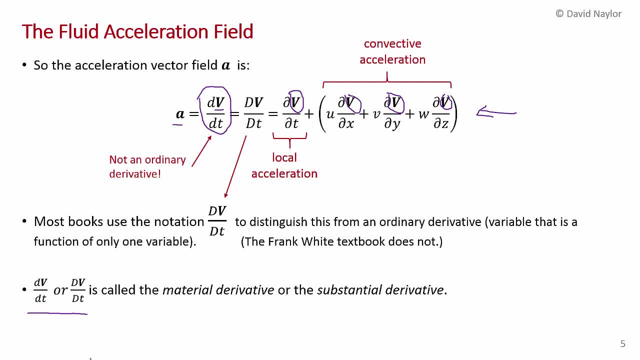 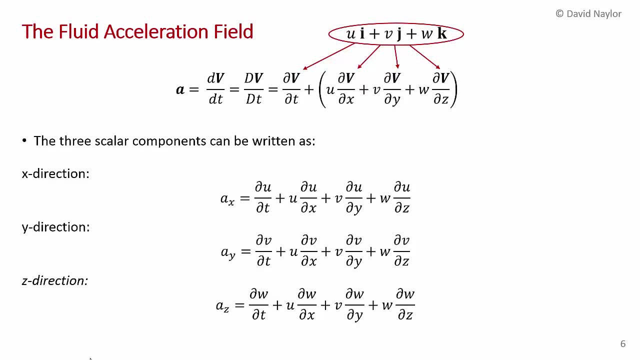 It's a little bit confusing in terms of nomenclature, but I think you can get used to it. So now we have the acceleration field and it's got this total acceleration that includes the local acceleration and the convective accelerations here. 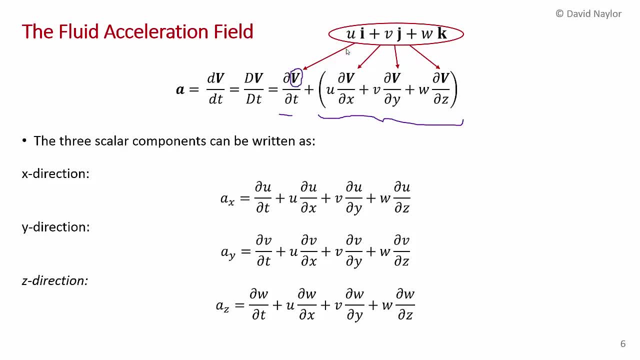 And what you've got to remember is this: velocity vector v has u in the i direction, v in the j direction and w in the k direction. So if you expand this, this equation out, and then you just pull off the i direction, 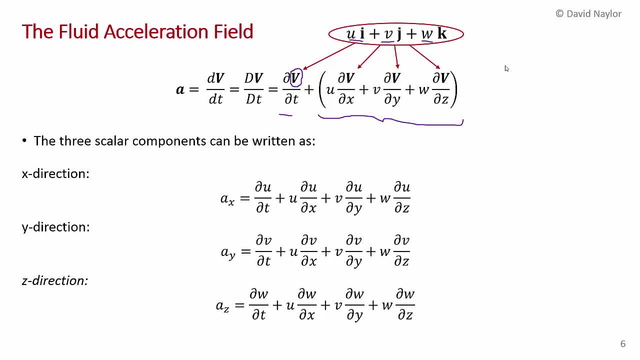 the. you know the x direction, you pull off the y direction, you pull off the k direction. what you get is the three components of acceleration. These are the scalar components of acceleration in the x, y and z direction. So acceleration in the x is di u, di x u di u, sorry, di u di t. 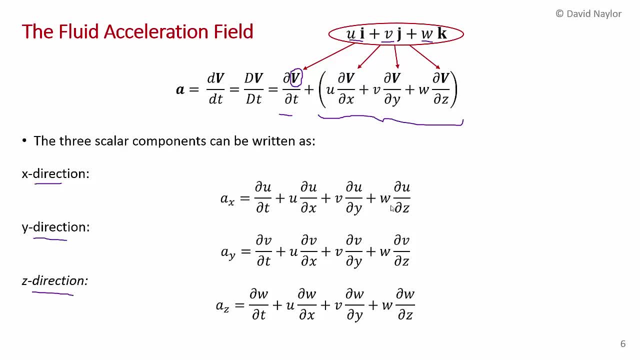 u di t, di x, v, di u di y, w, di u di z, And similarly in the y direction we have the local acceleration in the v direction, so that's caused by the transients in the flow and then the convective accelerations. 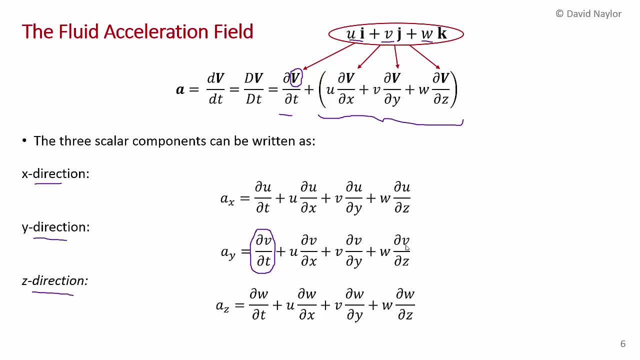 But here now we've replaced, we have v, but the rest of the form remains the same. So u di v di x, v, di v di y, w, di v di z, And you can see the form remains the same. If you look at the accelerations in the z direction: 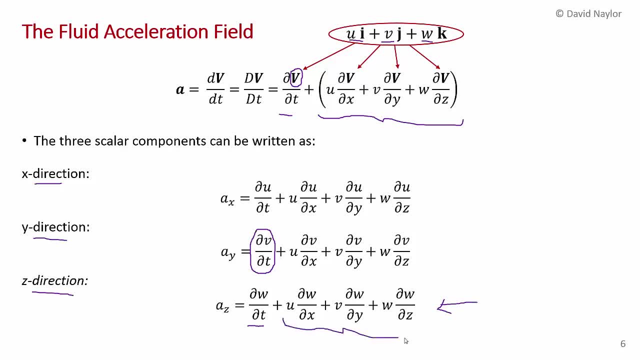 we have the local acceleration and the convective accelerations, but now we have w in here. It's worth- I don't want to say memorizing, but it's worth using these equations enough that you get comfortable with those forms. Now this next slide. I almost hesitate to mention it. 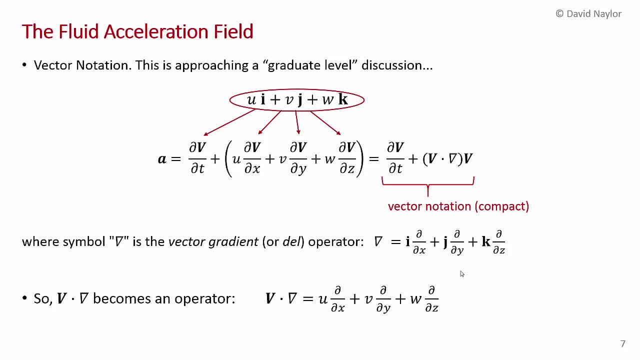 It's really approaching a graduate level discussion of this. But you'll see this acceleration, this substantive, derivative form of the acceleration field, you'll see it expressed in vector notation and the vector notation is shown over here. So it just becomes v di t, where v is the vector. 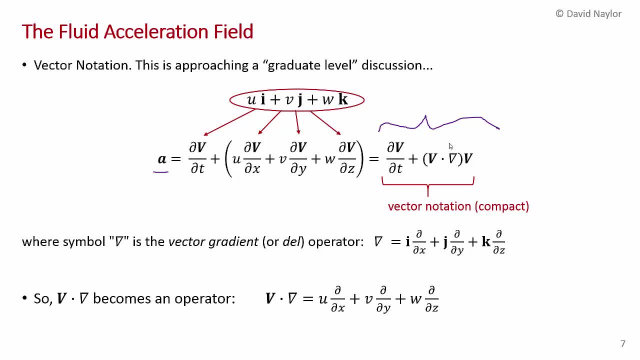 and then v dotted into this upside down triangle which is the del, and then that becomes an operator that acts on the velocity vector. So remember, this del or gradient operator is i, di by dx, j, di by dy, and then y, k. 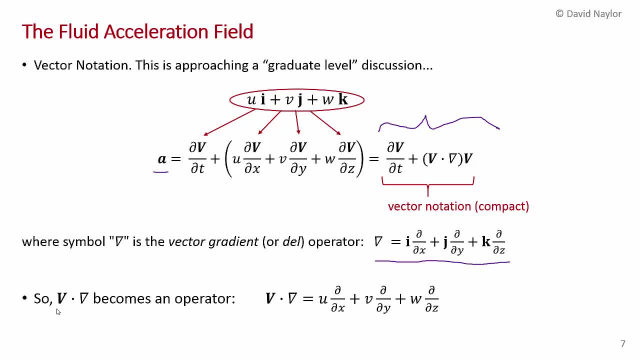 v di by dy z. So if you imagine v and a dot product of the velocity vector and the del operator, then that becomes u di by dx, v di by dy y, w di by dy z. And if you operate that you apply that operator to the vector field v. 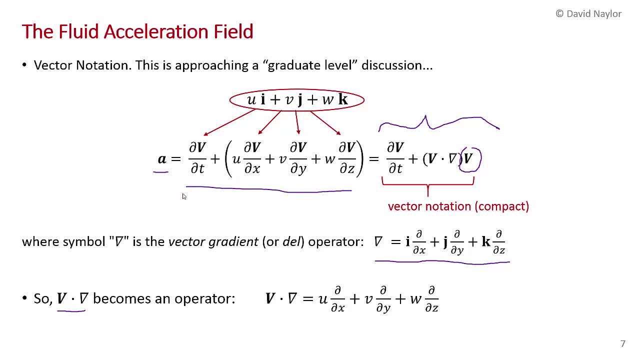 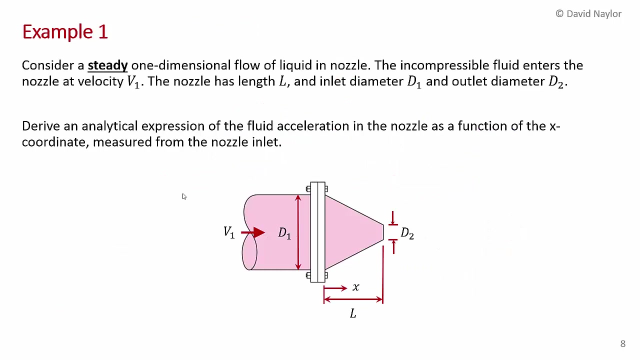 which has the three components, you recover the longer form of the acceleration expression. I show you this because many books, many papers just write it down in the vector form and it can be a little confusing if you've never seen it before. Now I'm going to do a couple of examples. 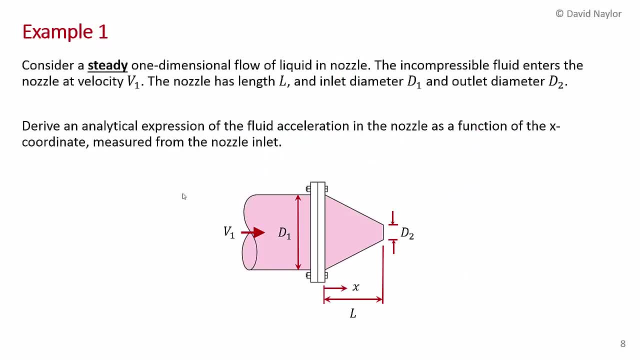 We're going to start with example one that considers steady, one-dimensional flow of liquid in a nozzle. So we're considering an incompressible fluid that enters a nozzle at velocity v1, and the nozzle has length l, has diameter, d1 at the inlet. 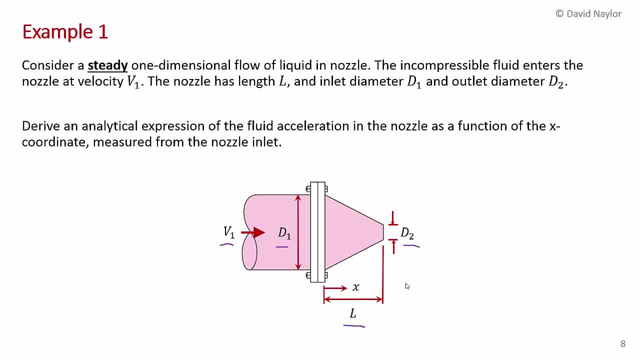 and diameter d2 at the outlet, And we're asked to derive an analytical expression for the fluid acceleration as a function of x, where the x coordinate here is measured from the nozzle inlet, And here of course we only have convective accelerations. 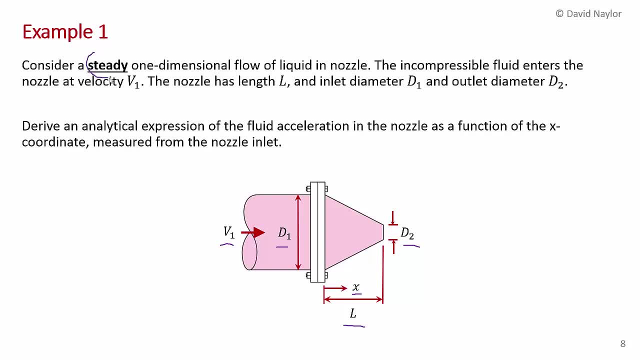 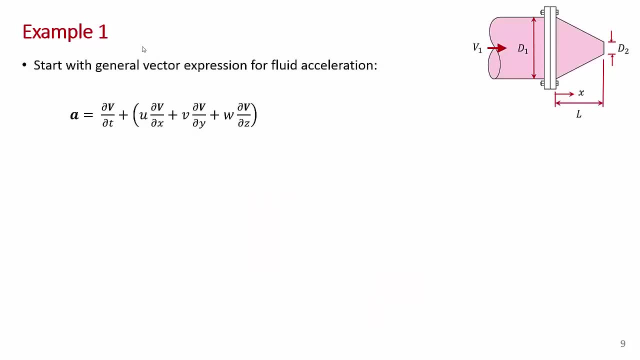 because we're dealing with. it says in the problem. we're dealing with a steady flow. So let's go through the details of this. We start with the general vector expression for acceleration. So here's the acceleration vector bolded, There's the local acceleration. 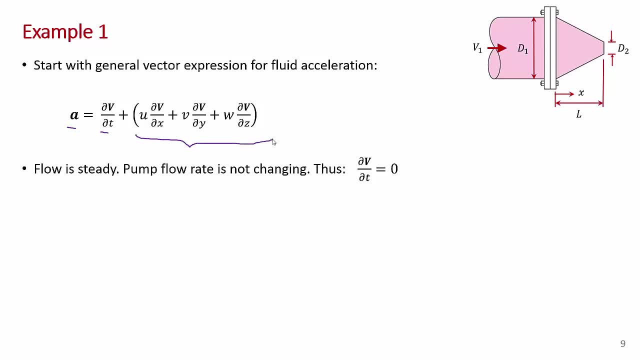 and then these are the convective accelerations, And it's mentioned in the problem that the flow is steady. the pump flow rate's not changing, so di v di t is zero. We have no local acceleration, You're told in the problem. 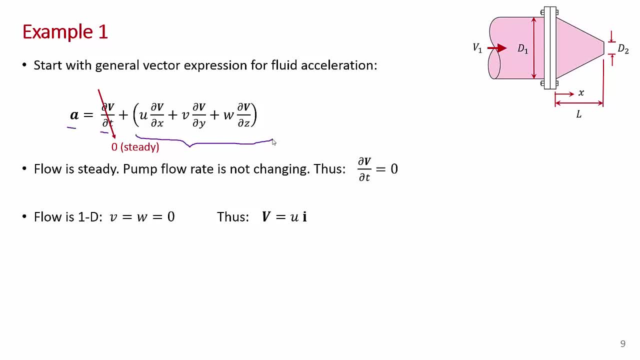 the problem. to approximate, the flow is one-dimensional, So v and w, the y component and z components of velocity are zero. So our velocity vector just has one component. v equals u in the i direction, And so v and w are zero. 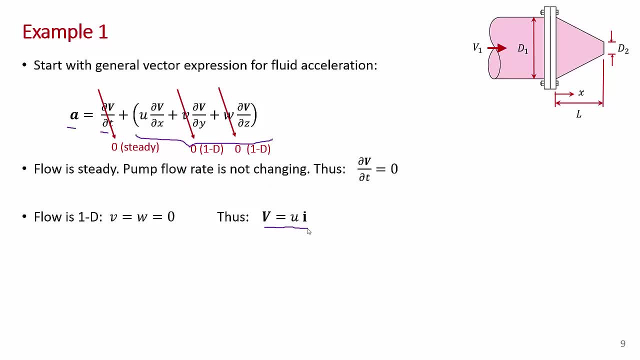 The derivatives di v di y and di v di z are also zero. So those terms go away, And so our acceleration equation. we only have acceleration in the x direction, and it becomes: the acceleration in the x direction is just u di u di x. 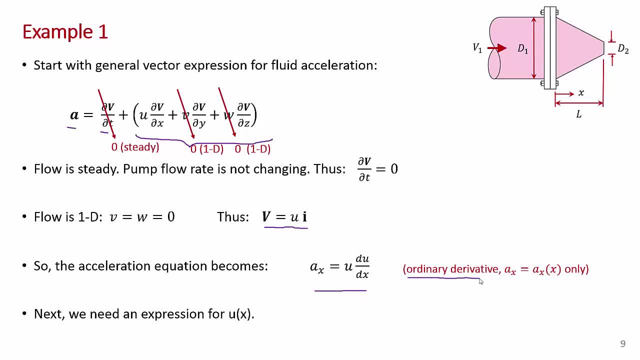 Notice. now I've replaced these with full derivatives. That's an ordinary derivative in this case, because now our acceleration is only a function of the x variable. So now to get an analytical expression for the acceleration in the x direction, we just need to get an expression for how the velocity varies in the nozzle. 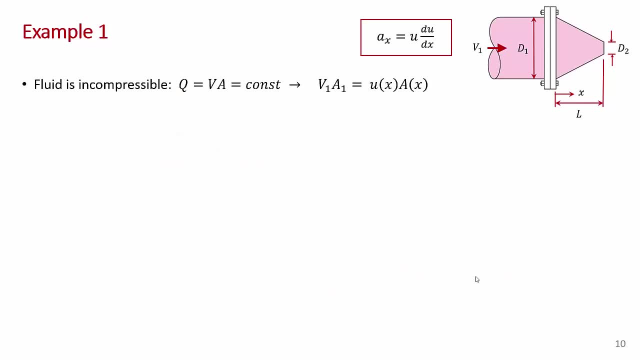 And that's pretty straightforward. We can do that using the concepts from the previous chapter. We know the flow is incompressible. it's a liquid, so the flow rates a constant, VA is a constant, so using V 1 and the cross-sectional area 1, that's got equal the velocity at. 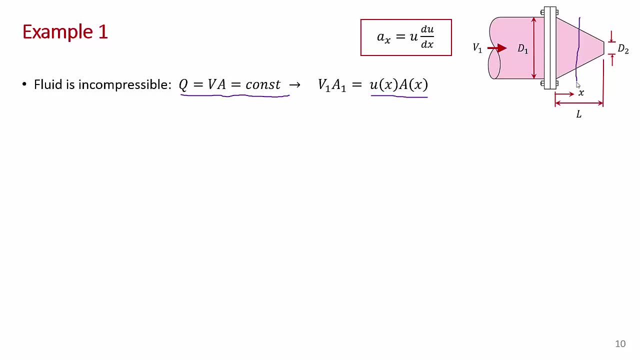 any X location in the, the nozzle times, the cross-sectional area at that cross-section in the nozzle. so we can solve for for UX. so I just solved here for for for UX and we get that it's a 1 V 1 over a of X, where a of X is the. 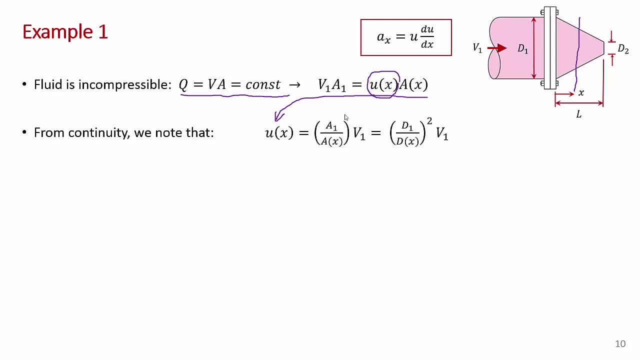 cross-sectional area. now the cross-sectional area is of course pi times the local diameter squared divided by 4 pi and the 4 is going to cancel, so we're going to have that the local velocity varies as D 1 over DX, the D of X squared times V 1. we can see from the image that 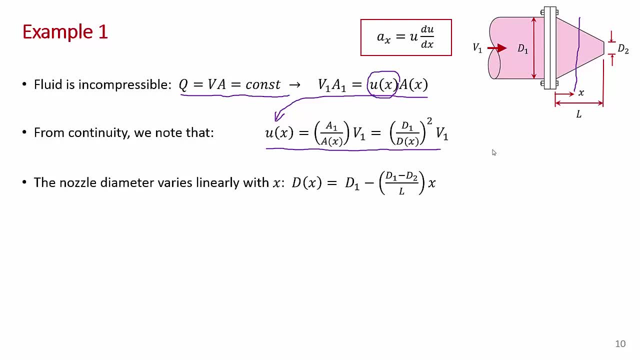 they're not going to be the same, so we're going to have that. the local velocity varies as D: 1 over DX, D of X squared times V: 1. we can see from the image that they nozzle diameter varies linearly with distance X. so we can write the: 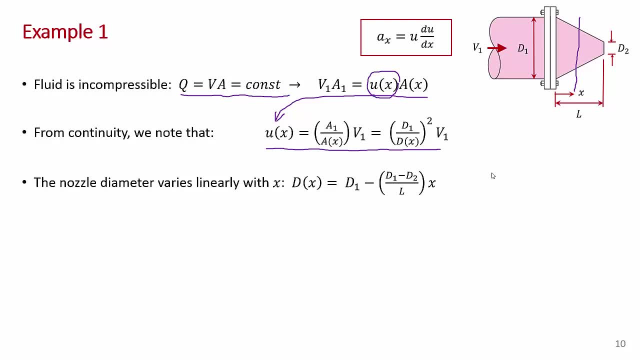 expression that D of X equals D 1 minus D 1 minus D 2 over L times X. you can check this is correct, because if you put in here X equals 0, of course you recover D 1, and if you put in X equals L, you recover D 2. if you put in L here, you 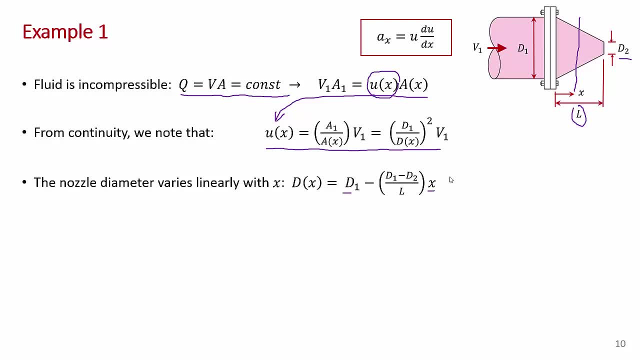 get D 1 minus D 1 plus D 2, so you get D 2. so that's you can see just by inspection that that linear equation is correct. so now what I'm going to do is substitute this expression for the diameter into into the expression for velocity, and so that's what's been done in this. next, 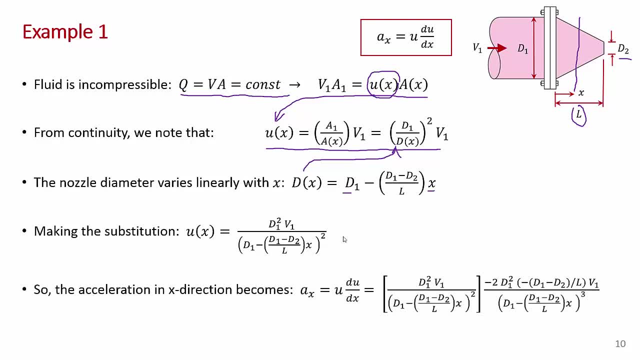 equation. so now we can actually start to evaluate our acceleration, because we previously we showed that the acceleration was only convective in the X direction and it's U to U DX. so the acceleration in the X direction is U to U DX. this is, this is our 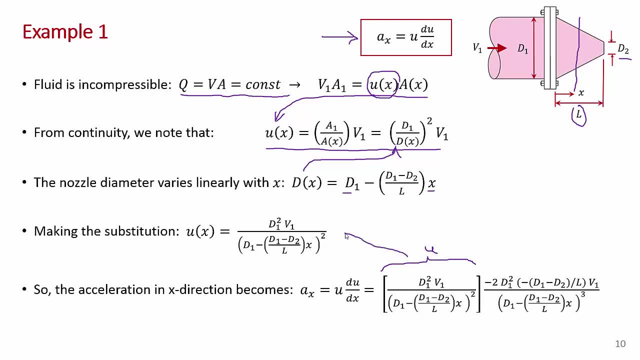 expression for U. so I've just made the substitution there. so D squared, V 1, and then D 1, D 1 minus D 2, L, X, all squared. so you can see that that's been just a simple substitution. and now this term here is D, U, DX, right. 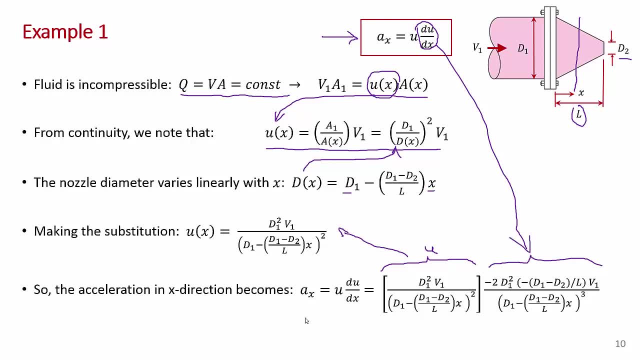 so let's just check that derivative. so keep in mind that X appears on the bottom, so that's like X, so that's that exponent. there is minus 2, so when we take the derivative we're going to have minus 2 times the entire expression here. 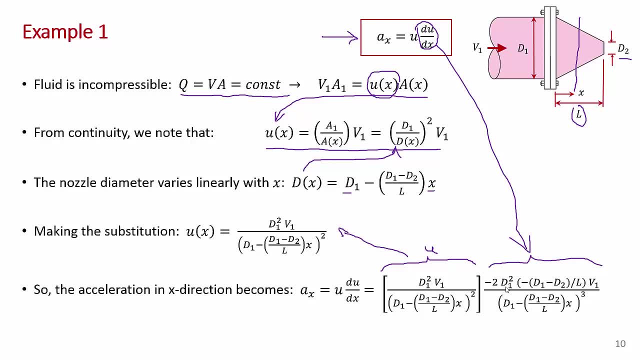 you can see it: minus 2, D 1 squared V 1. I was over on this side and then, and then we repeat the bottom. but because we've taken the derivative, that becomes a minus 3 and now we have to take the derivative of the expression. 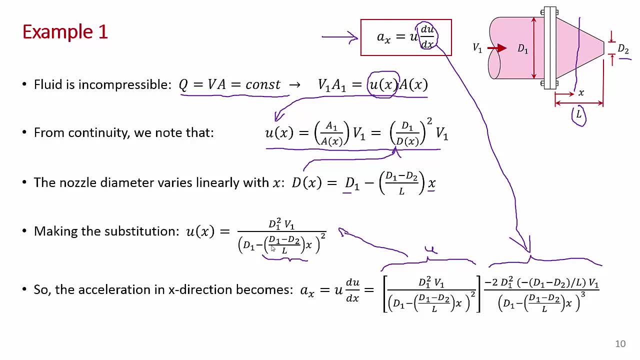 on the bottom inside the exponent, and so we get minus D 1, minus D 2 upon L. so that looks correct to me. now in the next slide, I think I've made a little simplification here. of course we have a minus and a minus, so the minus sign. 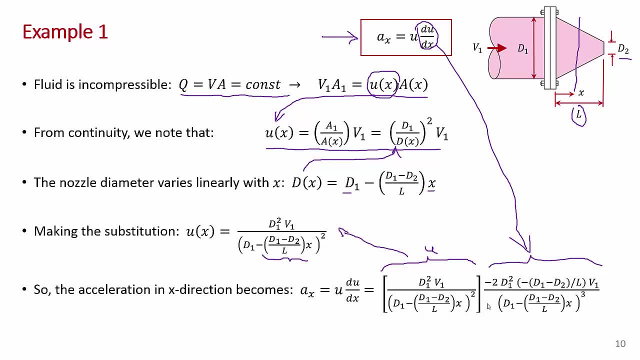 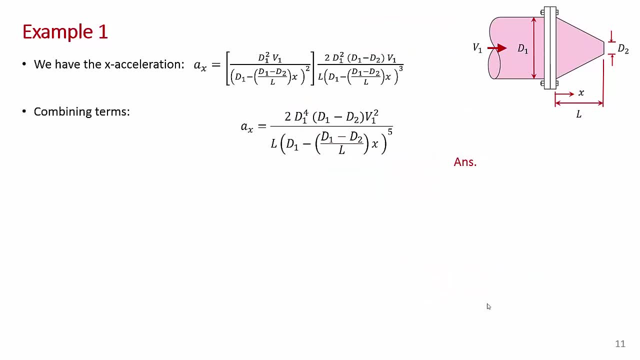 disappears. I brought the L down on the bottom. so let's just rewriting the expression that we obtained in the previous slide with a little bit of simplification: getting we're getting rid of the two minus signs to make a plus sign and bringing the L here down on the bottom. now I can. 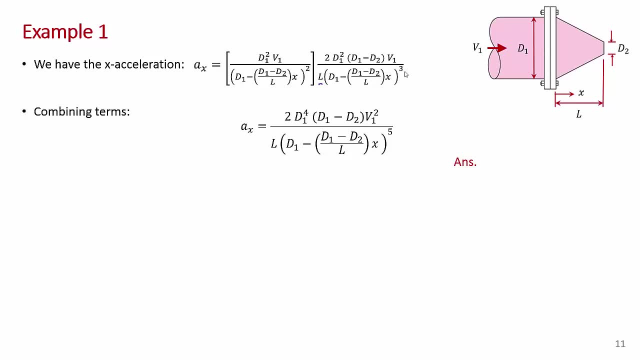 combine terms. we've got the same term here squared and the same term here cubed, so that becomes this term becomes to the fifth power. I can combine the D ones and the D one here becomes D 1 to the fourth and the V 1, V 1 becomes. 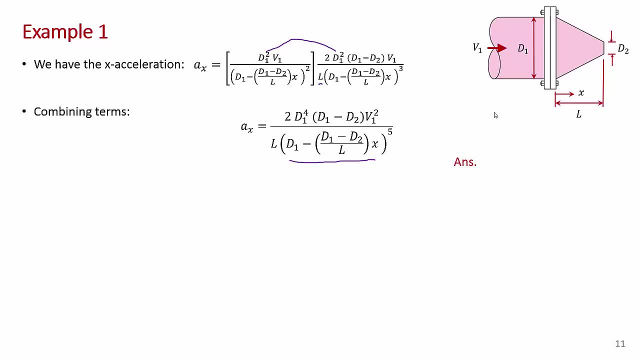 a V 1 squared, and so that's our final answer. it's always good to check the units. it's not 100 percent foolproof, but it's a good way to check that you haven't accidentally dropped a term. so of course, we have D one. 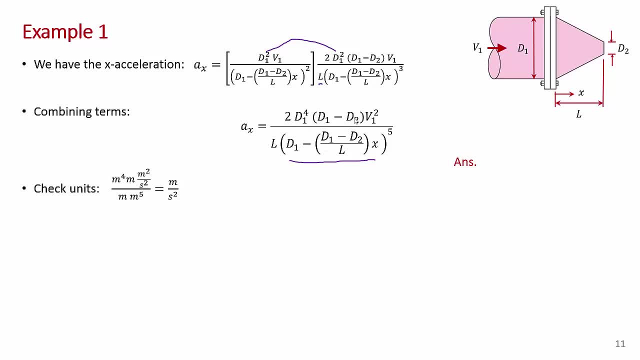 is meters to the fourth, and then this term, D 1 minus T 2, is going to have units of meters. velocity 1 squared is meters squared per second. squared L has units of meters and this term, of course, is going to have units of meters to the 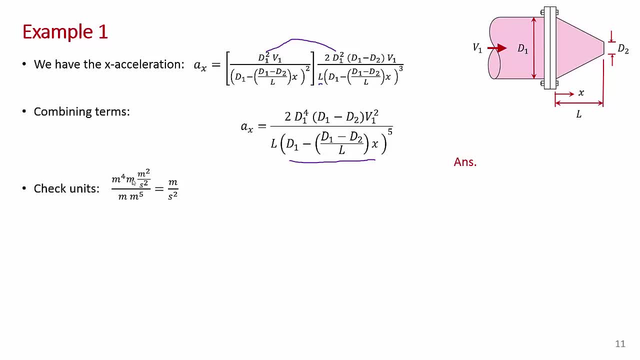 fifth, and so we can see here that that's meters to the fifth, meters to the fifth, that meter goes with that meter and we have meter per second squared, which is correct units for acceleration. I'll end this example just by making a couple of comments. if you look at this expression, you'll see that the acceleration is: 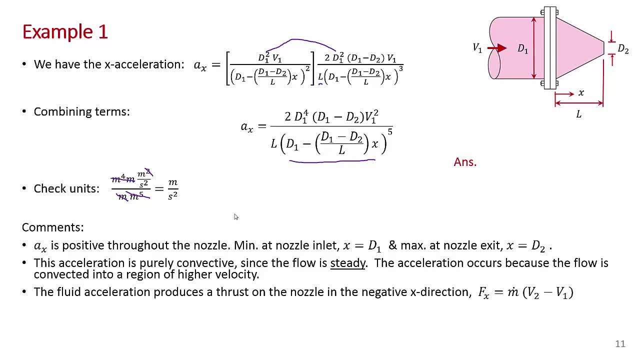 positive throughout the nozzle. if you try evaluating it, you'll see that the minimum acceleration is at the inlet to the nozzle, at d1, and the fluidic acceleration increases to a maximum at the exit plane, d2. I mentioned previously that this acceleration is purely convective. there's the since the flow is. 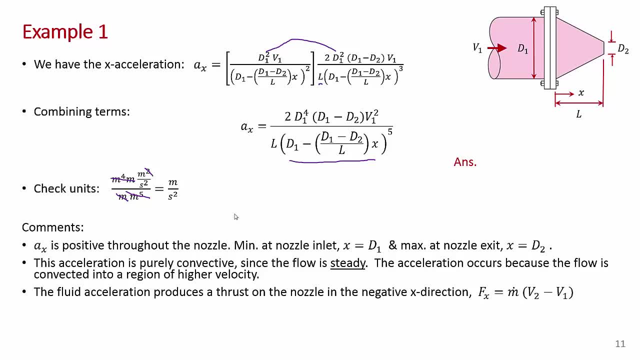 steady, there's no local acceleration and the acceleration occurs because the flow is being convected into a region of higher velocity. and just as an aside, we saw in the- the previous chapter where we were calculating forces from impulse momentum, that the acceleration of the fluid through a nozzle actually produces a 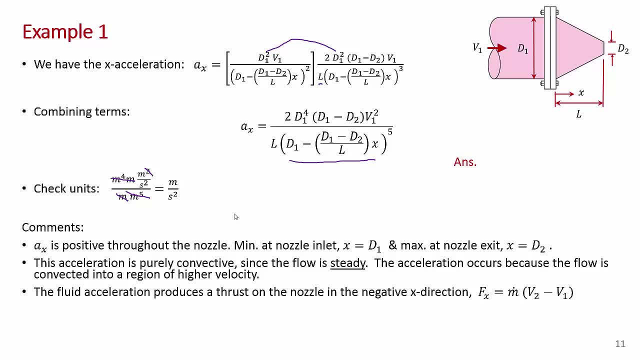 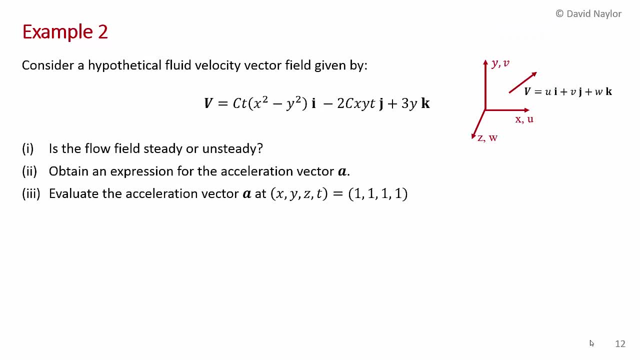 thrust on the nozzle in the negative x direction. so I'll end with this example. what we're considering here is a hypothetical fluid velocity vector field given by the following expression: so we have the velocity vector V here, given by c, t, x squared, minus y squared in the i direction. that's the velocity. 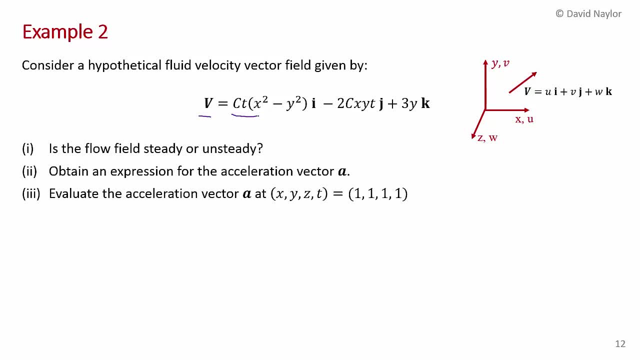 vector component in the x direction. so this we normally denote as u lowercase u. we have minus 2 c, x, y, t in the j direction or in the y direction, so this we normally denote as lowercase v plus 3y in the k or z direction. so this we denote: 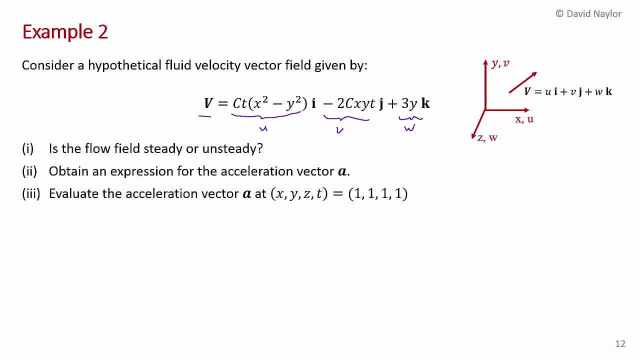 as the velocity component w. and so, given this velocity vector field, we're asked: is the flow steady or unsteady? then we're asked to obtain an expression for the acceleration vector- remember, bolded letters are vectors- and then, once we get that expression, we're going to evaluate. 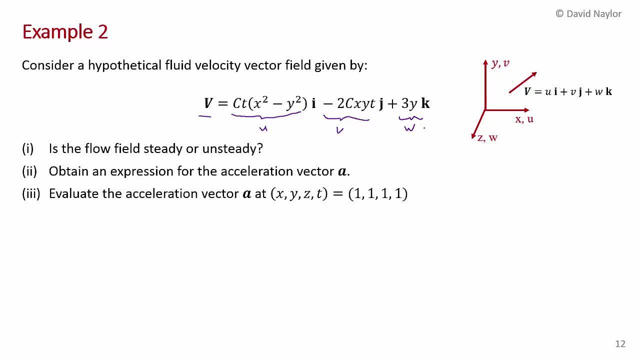 the acceleration vector at x, y, z, t equals 1, 1, 1, 1 where the units are arbitrary. so we start by considering the issue of steadiness or unsteadiness also. another way to express it is whether the fluid velocity field is transient and what we notice right away. 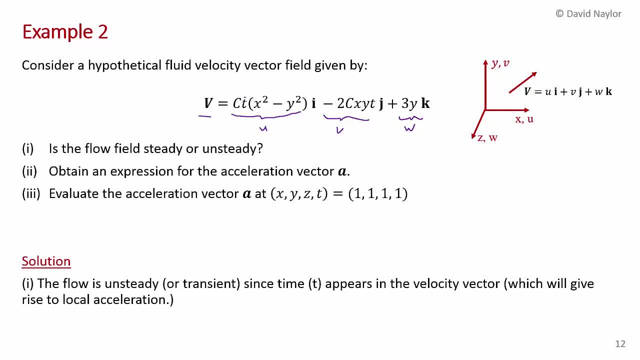 you look at, these is the U component and the V component of velocity, have time appearing in them, and so that's going to give rise to a local accelerations, and so the fact that time appears in just even one of the velocity components tells you that the velocity field is unsteady, or the velocity field is. 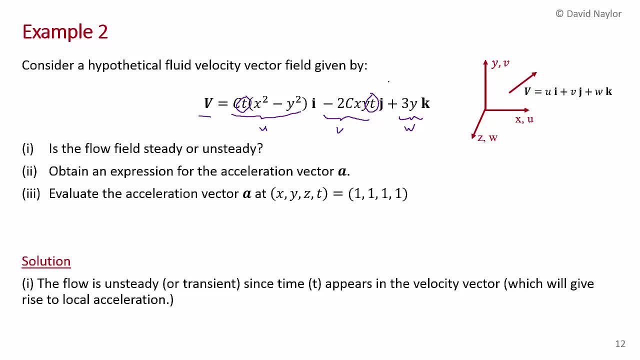 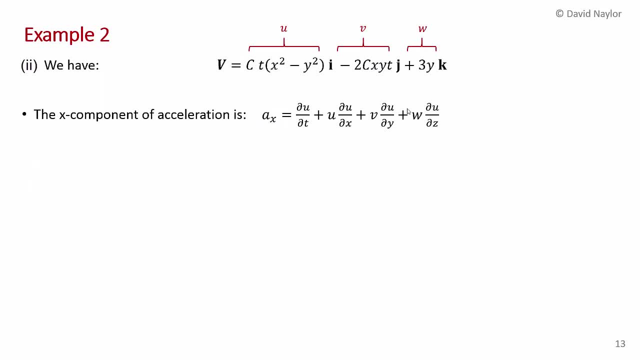 transient is another way to express that. for part three were asked that, given this velocity vector field, to derive the acceleration vector. so we're going to do this component by component. so the X component, as we just talked about, is di U di T, U, di U, di X, V, di U, di Y, W di U. 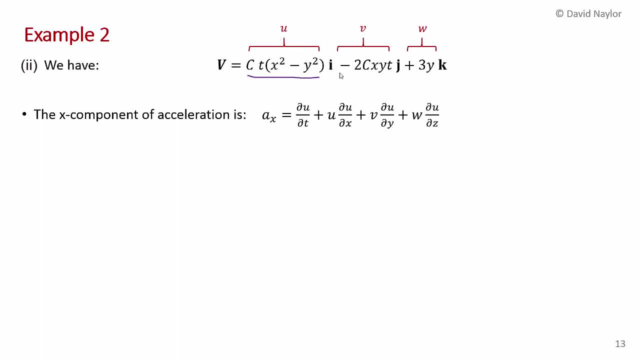 di Z, where- and I've shown here that this is U, this is V and this is W, so now we can evaluate these terms. so what we're evaluating here is di U di T, which is going to treat all the other variables as a constant when taking the. 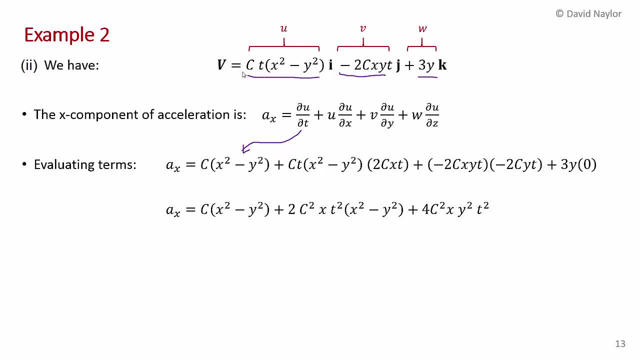 partial derivative with respect to time, so that's just going to become C X squared minus Y squared. then the next term is U di U di X. so I've rewritten U here, right. so C T X squared minus Y squared. and now I want to take the derivative of U with respect X, which is going to: 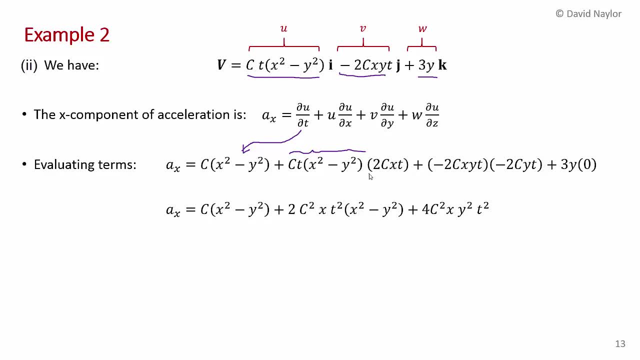 become 2 C, T, X. right here. the next term is V di U, di Y, so I've rewritten V minus C, X, Y, T there, and now I want to take the derivative of U with respect to Y, so that's going to become minus 2 Y. 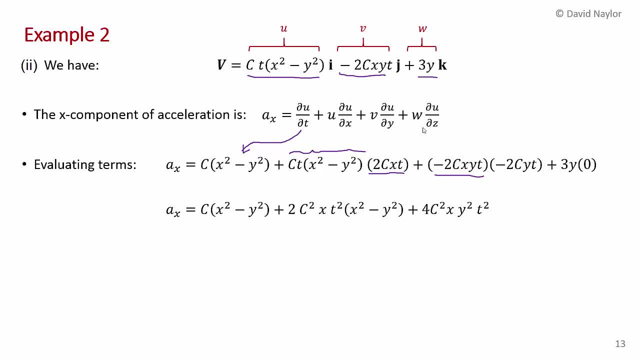 yeah, minus 2 Y, C, T, right, so there. and then finally we have W, di U, di Z, W. here is 3 Y, and then we take the derivative of U with respect to Z. there is no Z, so you're going to get 0. and then what I've done on the next line is just: 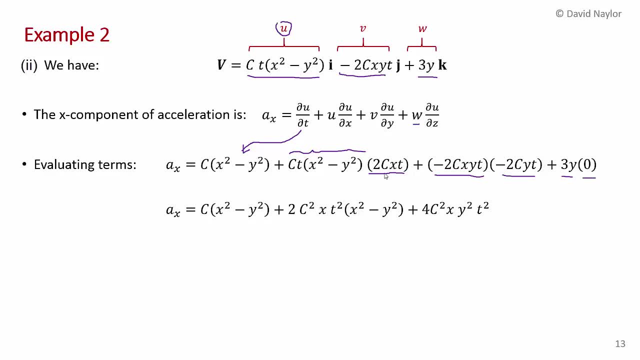 simplified this term here, so I brought the 2 out. so that's 2 C squared plus 2 Di, Z, Y squared. I square one times 2 X. there's T here and it T, there's what becomes T squared. yeah, that's. that's the simplified version. 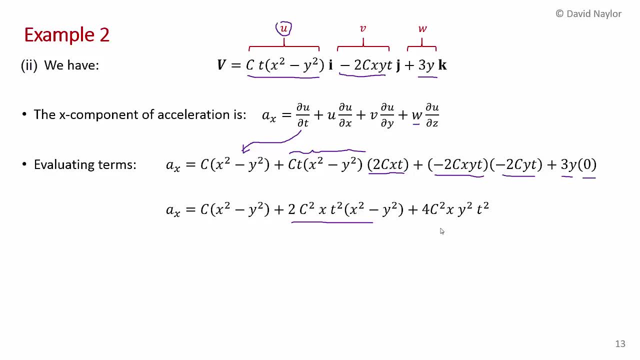 and then I've simplified this term: the minus and the minus give you a plus. so, and combining the C's and the Y's and the T's, we get 4 c squared, X, Y squared, T squared. that's just the acceleration in the X direction. we now have to repeat. 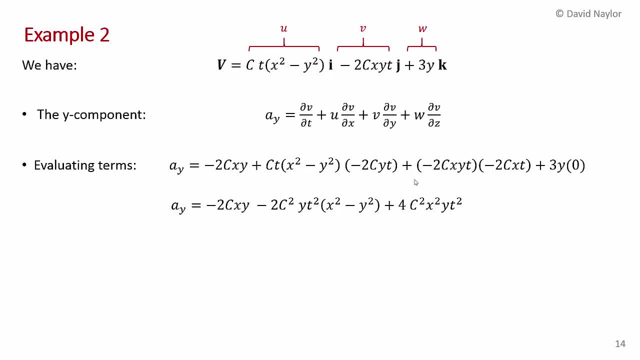 this for the Y and Z directions. Notice the form of the. there's the local accelerations, there's the convective accelerations, So di V, di T, U, di V di X, V, di V di Y, W, di V di Z. 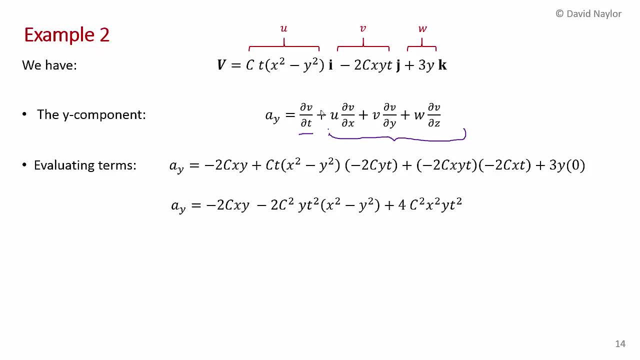 So now we evaluate these terms, Let's check this out. This is V here, So we're going to take di V di T first. That's going to become just minus 2CXY. Yeah, that's what we have. 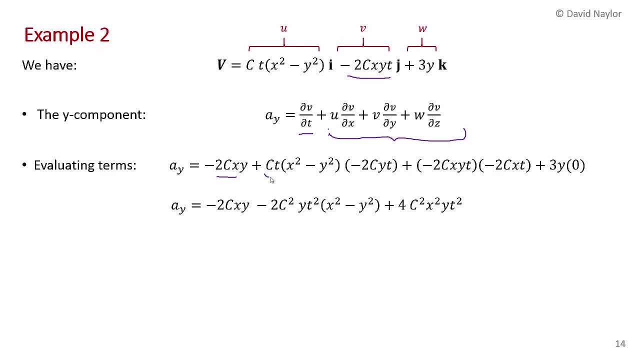 And then we take: I've reproduced U here, So here's U. That's correct. And now we want to take di V di X, So that's going to become minus 2CYT- Yeah, that's correct. And now the V di V di Y. 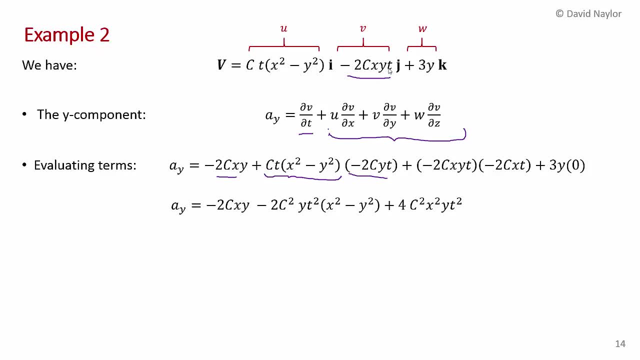 So I've rewritten V, which is minus 2CXYT, So that's V here. That's the V component, And then di V, di Y, So that's going to become minus 2CXT. Yes, that's correct. 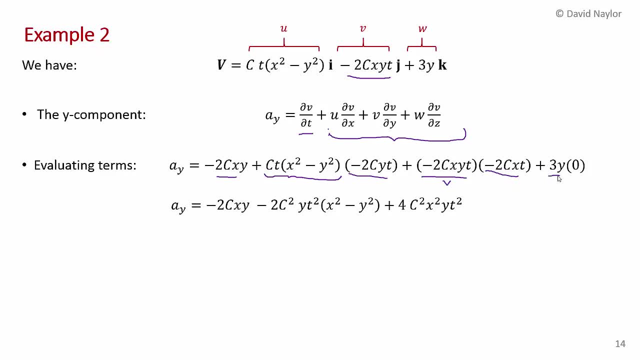 And then W again is 3Y. And then we want to take di V, di Z. Well, Z doesn't appear in V at all, So that gives you 0.. And then below- here I've just simplified This term here is going to become minus: C squared T squared Y. 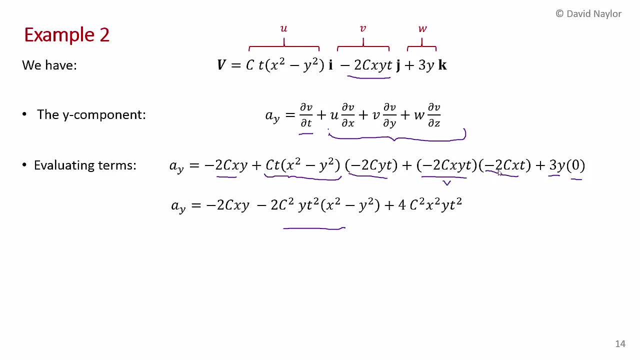 Right, That's correct. And then I've combined, of course, the negative signs. They become a positive sign And you get a 4C squared, X squared YT. Yeah, that looks correct too. Now we move on to the Z component of acceleration. 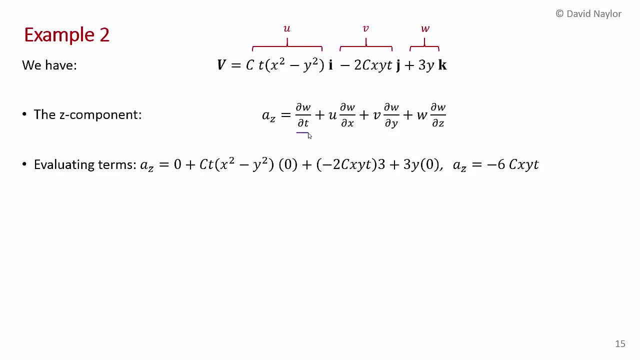 Again. now we're looking at the local acceleration, DW, DT, And now we have W in here. So it's U di W di X, V di W di Y, W di W di Z. So going term by term, keeping in mind that W is 3Y. 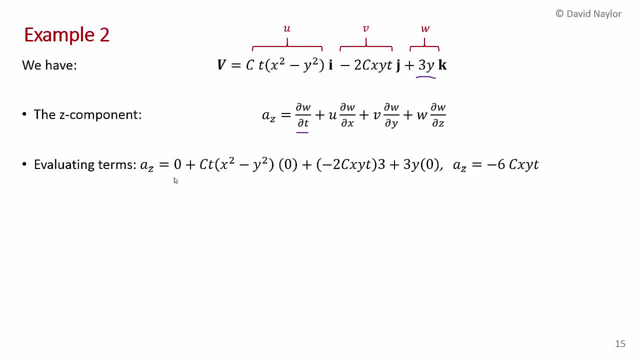 So if we take the derivative of 3Y with respect to T, we get 0.. Now I've rewritten U here. U is C, T, X squared minus Y squared. So there's U And then DW DX. 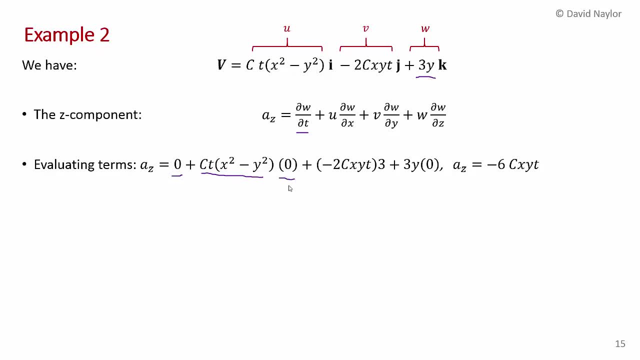 Well, W doesn't have X in it, so you get 0.. I've rewritten V here, minus 2CY or XYT. There's V. Of course, that was U And then times DW DY. Well, DW DY is just going to give you the 3.. 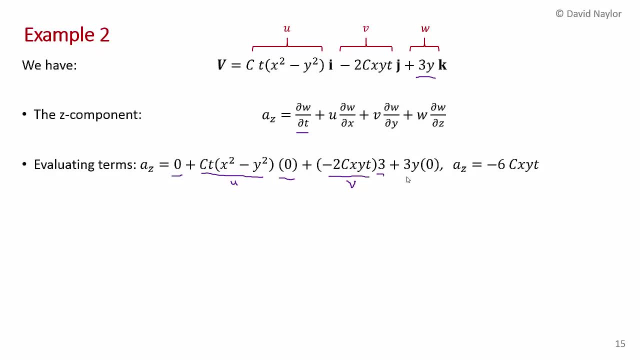 And then W, DW, DZ. Well, W is 3Y, And if you take DW DZ, W is 3Y, so it doesn't contain a Z. So that's going to be just a constant. give you a derivative of 0.. 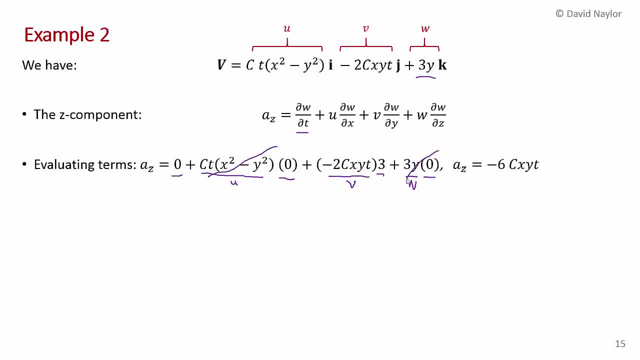 And so this term and this term will vanish and you only end up with minus 6CYXT. So now you've got the X, the Y and the Z components of acceleration. You can put them in as an acceleration vector. So this is just. 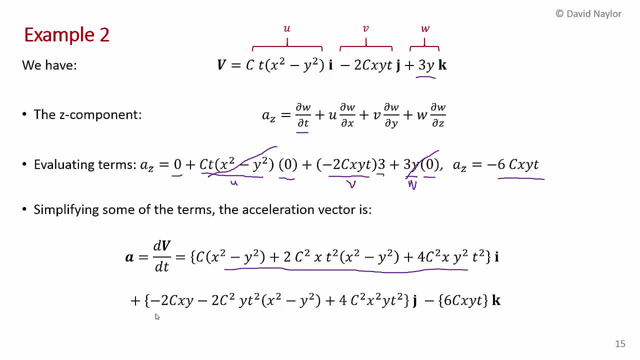 AX. a couple of slides back: AY, if you check back, that's AY And there's our AZ in the K direction. So that's the answer in terms of the general expression for the acceleration vector And on this slide I've just reproduced that expression at the top. 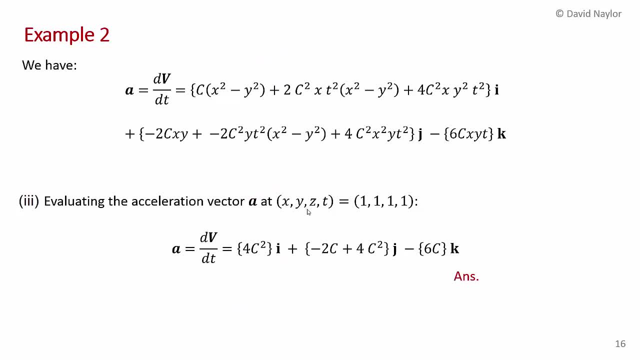 And you're just asked in the problem to evaluate this at XYZT. And you're just asked in the problem to evaluate this at XYZT. So you'll see if you look at this, this is 1 squared minus 1 squared.